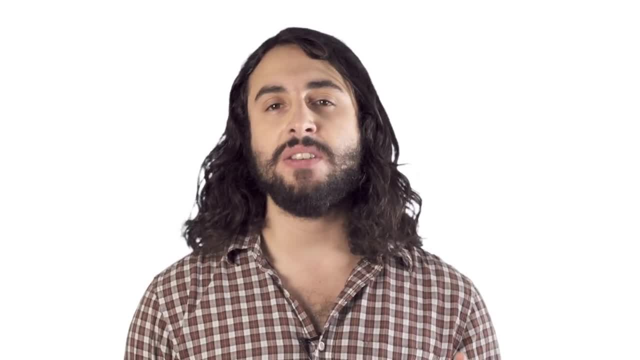 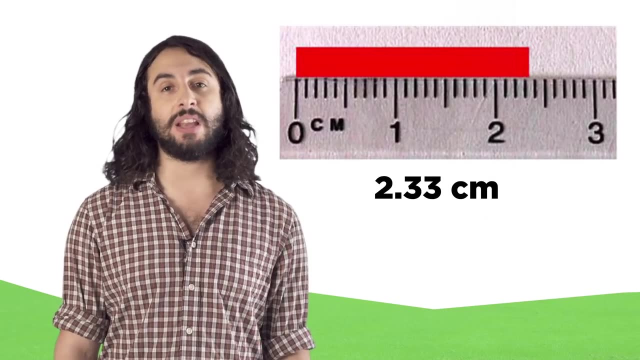 So when we use measuring devices we only estimate one digit further than the level of precision inherent in the instrument. Here we could estimate 2.33 centimeters, but not 2.33481.. We do not have access to that level of precision. 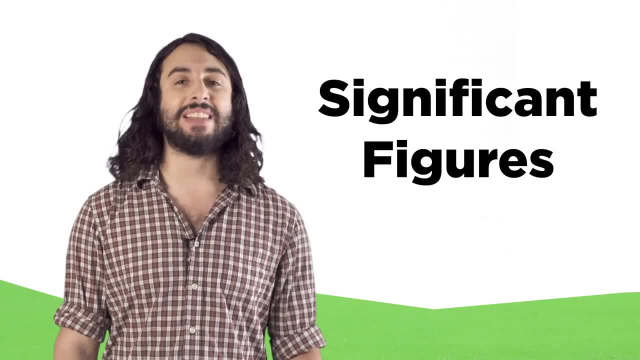 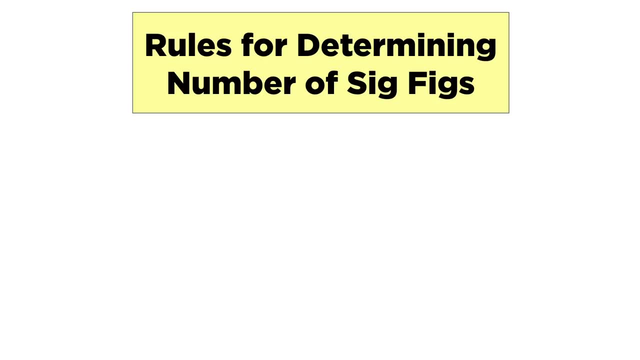 So any measurement will have a certain amount of significant figures, or sig figs, associated with it that display how precise it is. Here are the rules for determining how many sig figs are in a value: 1. Any digit that's not zero is significant. 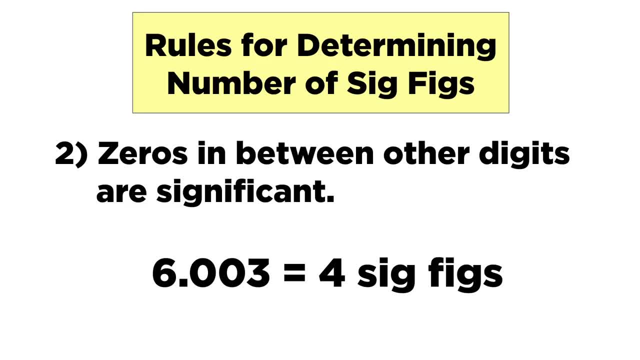 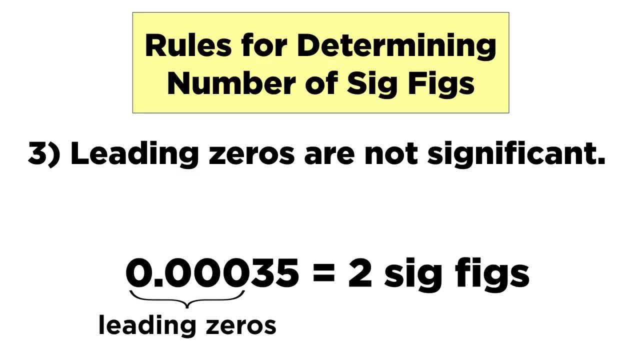 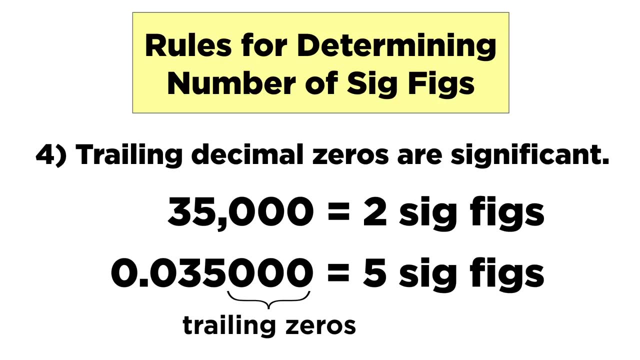 2. Zeros in between other non-zero digits are significant. 3. Leading zeros- ones that come before the first non-zero digit- are not significant. And 4. Trailing zeros: the ones that come after the last non-zero digit. 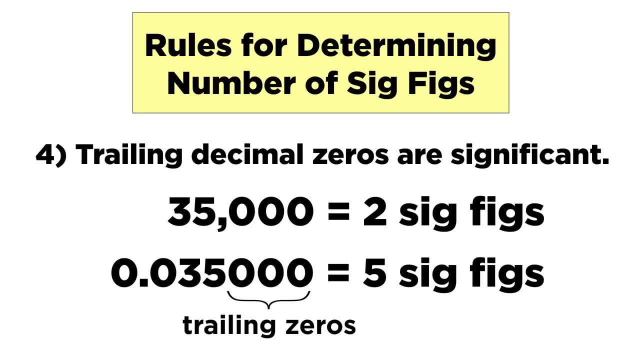 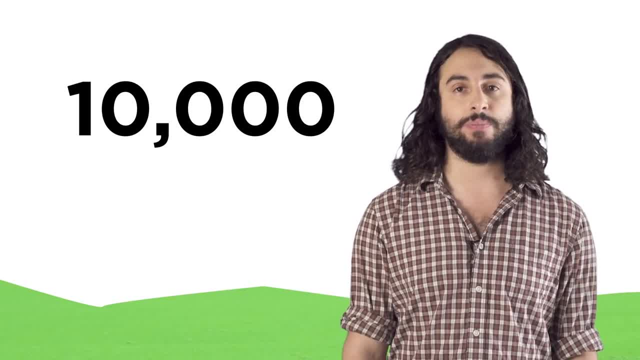 are only significant if they are decimal zeros. So 10,000 only has one significant figure, which really means it's about 10,000, not exactly 10,000.. If we bring back that same crowd and one more person shows up, can we estimate 10,001?. 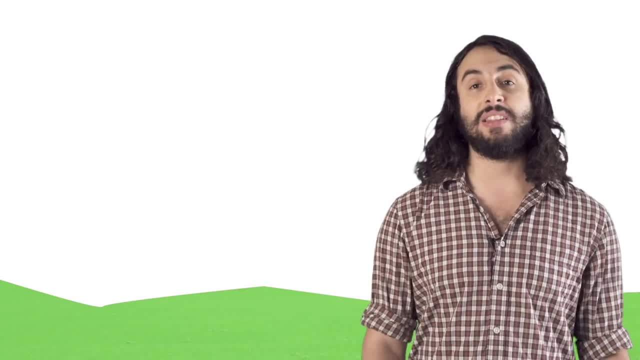 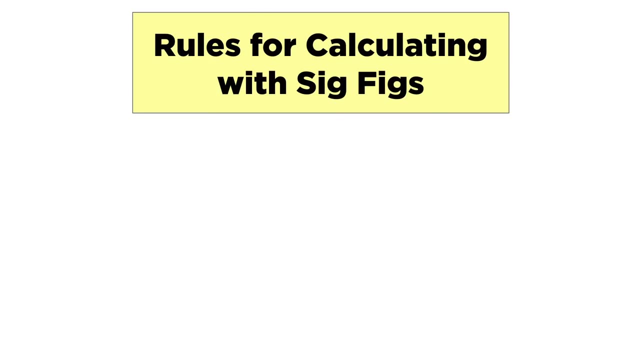 No, because we have only estimated to one sig fig. so anything from 9,500 to 10,499 would round to our estimate of 10,000.. When we do calculations we have to pay attention to the number of sig figs. 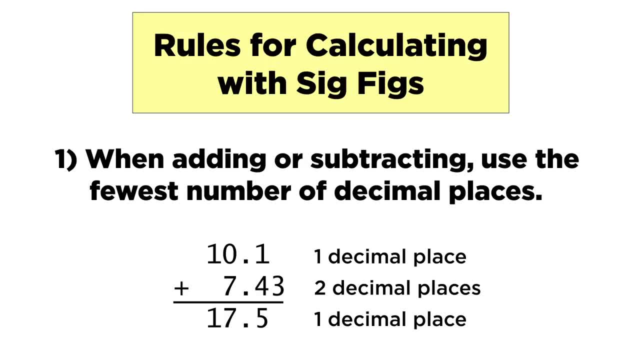 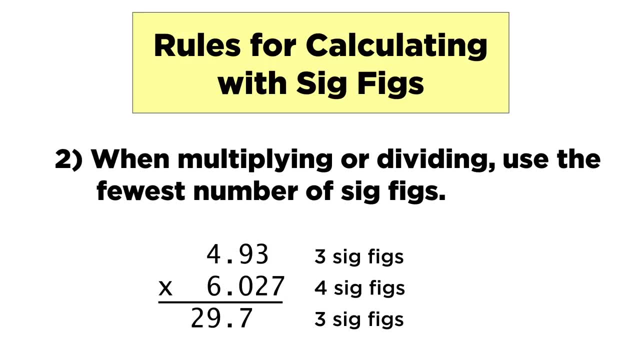 If we are adding or subtracting, our answer will have as many decimal places as the value with the least number of decimal places. If we are multiplying or dividing, our answer will have as many sig figs as the value with the least number of sig figs. 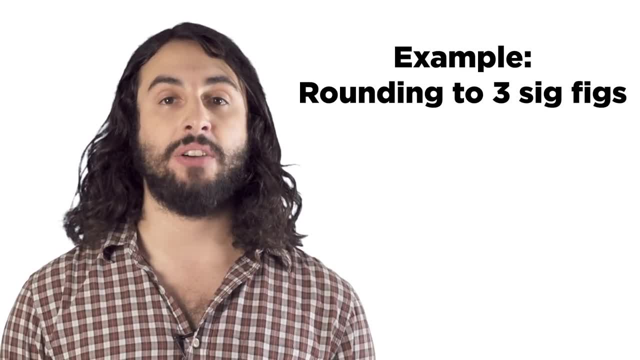 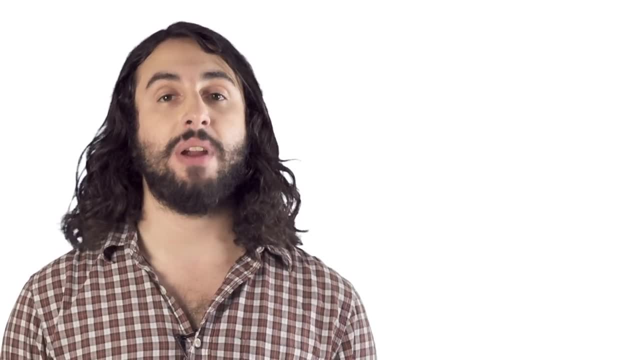 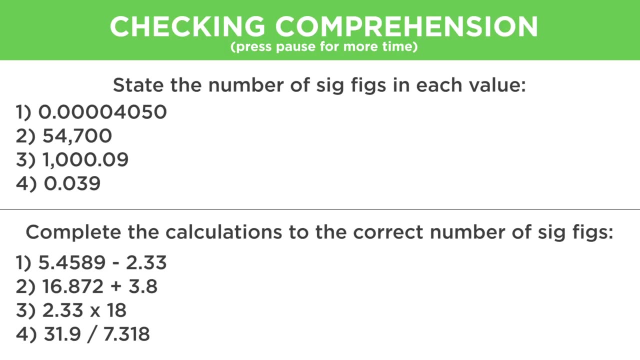 Whatever our answer is, we will have to round up or down at the appropriate digit. 5 or higher means round up, 4 or below means round down. Let's check comprehension. If we are able to round up, we will have to round up. 4 or below means round down. 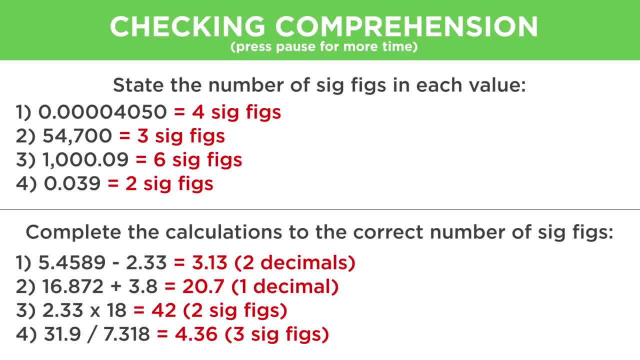 Let's check comprehension. If we are able to round up, we will have to round up. 4 or below means round down. If we are able to round up, we will have to round up. 4 or below means round down.